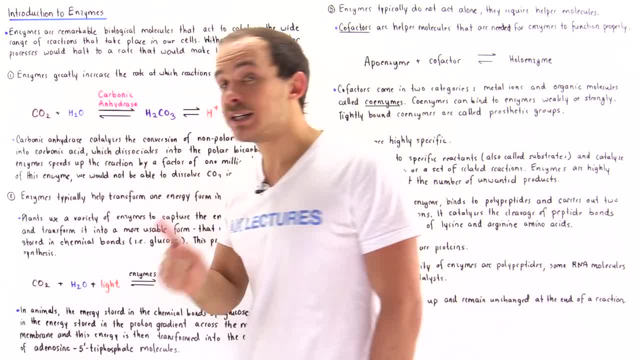 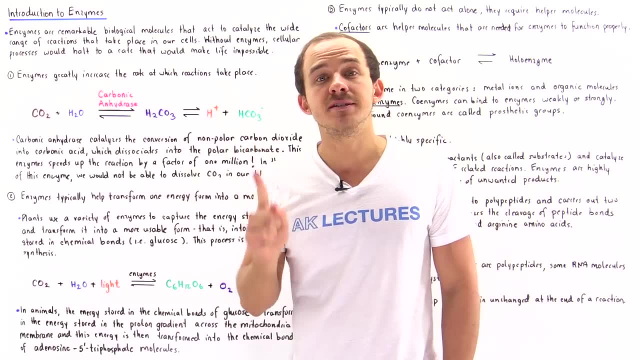 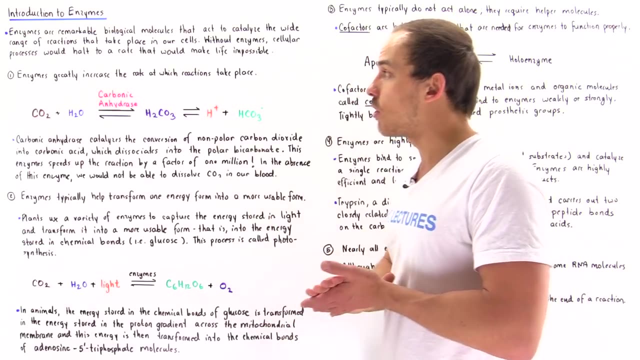 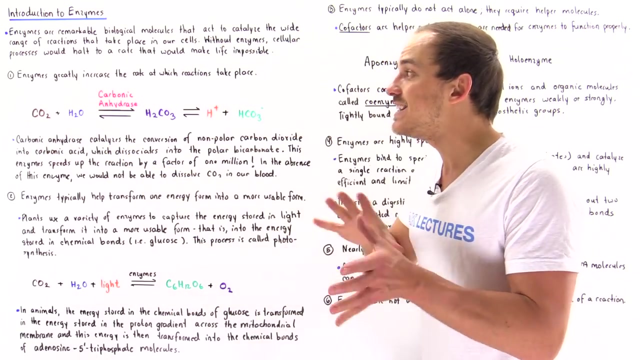 enzymes are. In fact, this molecule can convert. the enzyme can transform one way or another into a human form. Now, in nature, carbon dioxide is a very positive. There are five different solutions to this model. It's an NCadamente andare structure, which means that generations after generations carbon dioxide 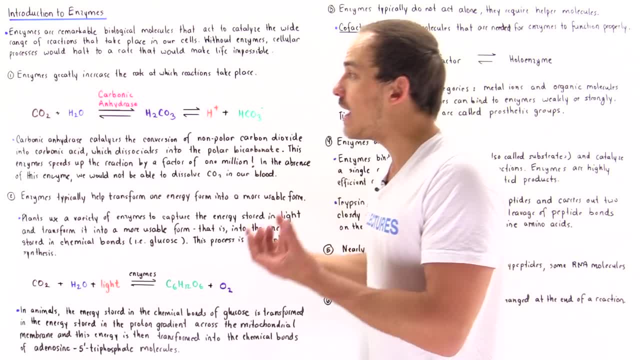 has an excretion and outer' increase within it's구 И Carbondioxide molecules every single second. So It increases the rate by one million. compared to its uncatalized formand creates uncadalyzed molecules: Nucleoca신, Clso дела. 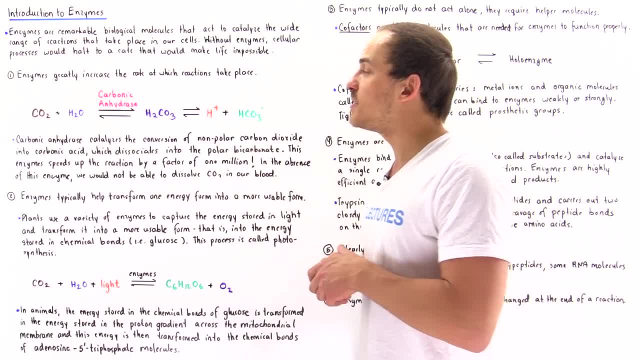 This enzyme basically helps us the nonpolar carbon dioxide that cannot dissolve inside our blood into a form that can be dissolved inside our blood, And that's precisely what allows us to from the cells and eventually expel it by the lungs of our body. Now, fact number. 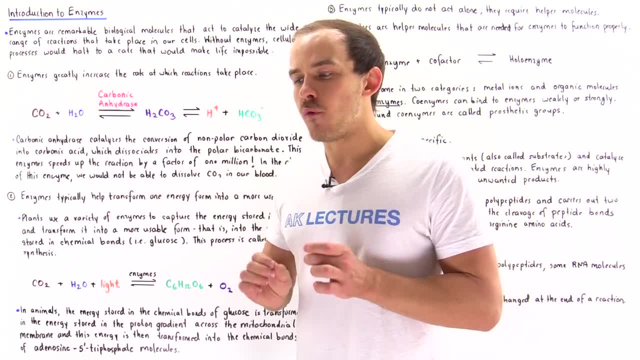 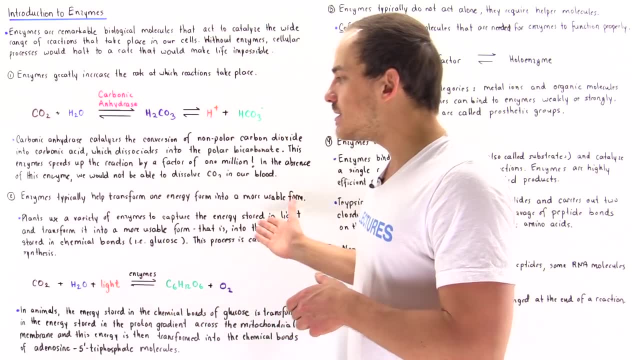 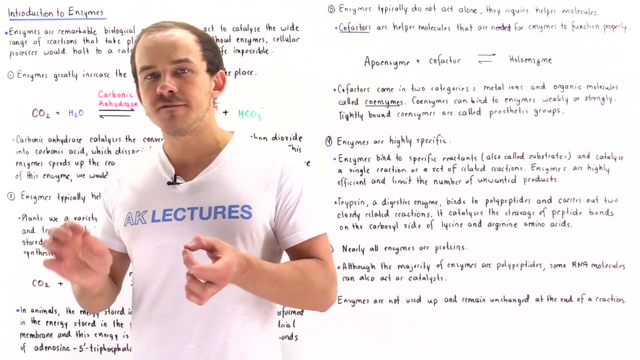 two about enzymes. Enzymes typically transform one form of energy into a much more useful form of energy, and one example is the process of photosynthesis, which takes place in plants. So inside plants we have a variety of different types of enzymes that essentially transform, They harvest or capture the 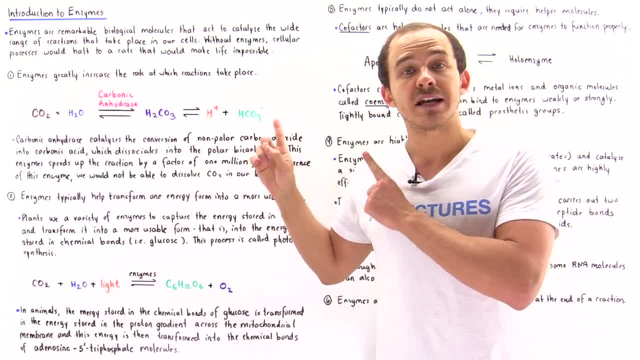 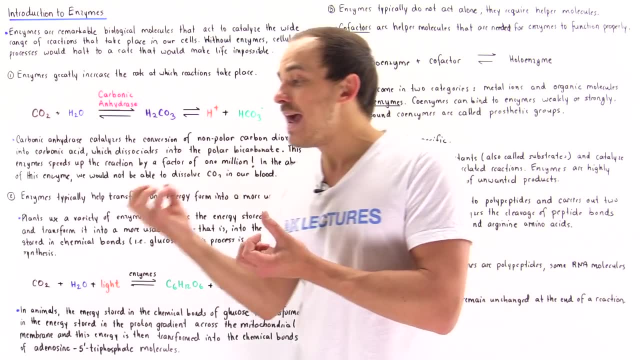 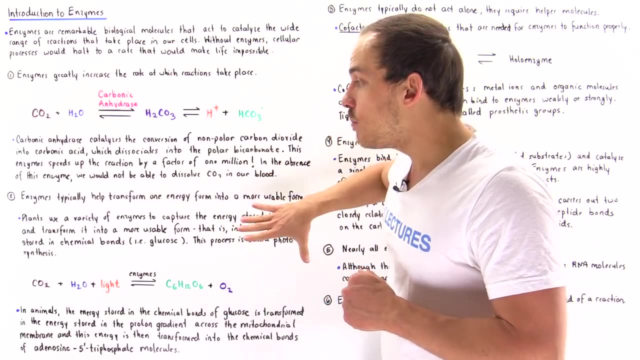 energy that is stored in electromagnetic radiation that comes from the sun, namely light. So they transform the energy that is stored in light into energy stored in a chemical bonds of glucose and sugar molecules. Now humans and other animals then eat that glucose and they themselves use. 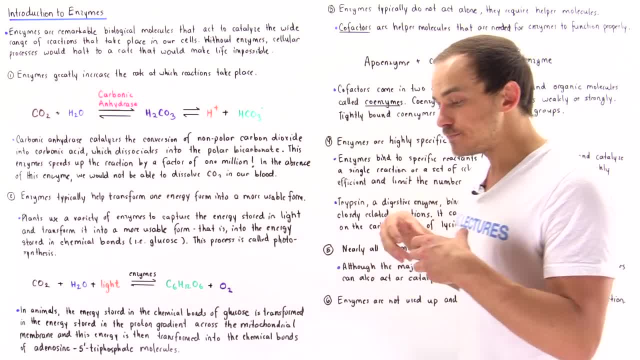 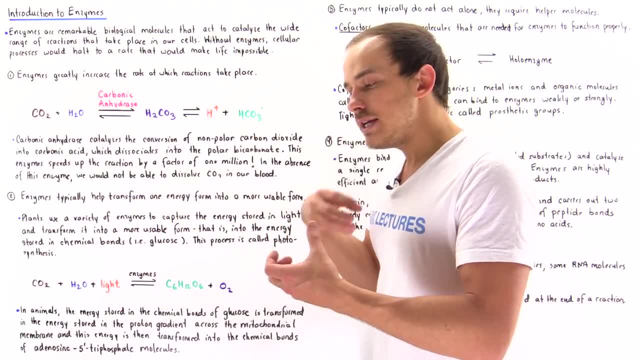 enzymes and in the process we're going to discuss eventually the processes glycolysis, pyruvate decarbonization, beta-carotene, beta- dismissive iron production and so on, carboxylation and then the Krebs cycle. So basically, in these processes we have many. 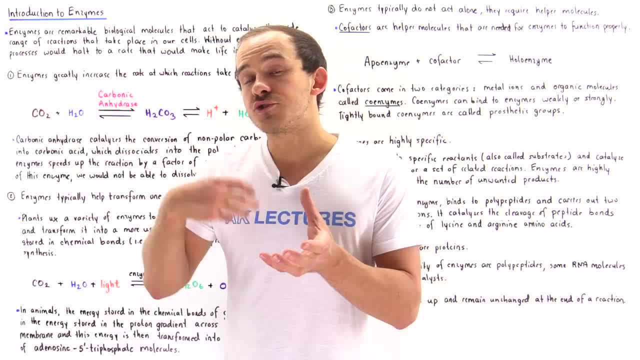 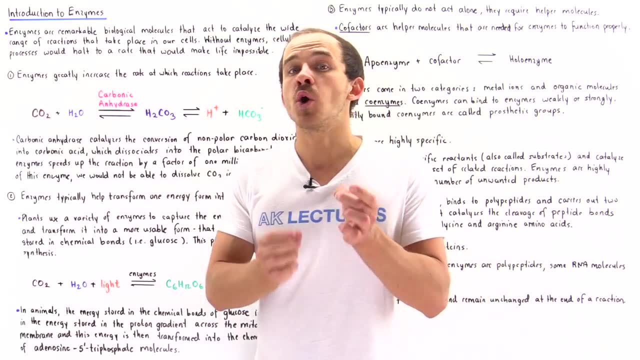 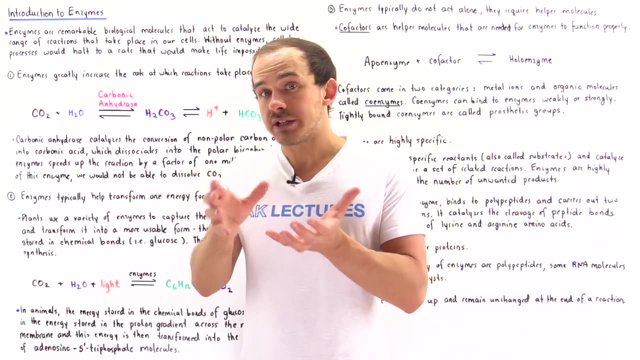 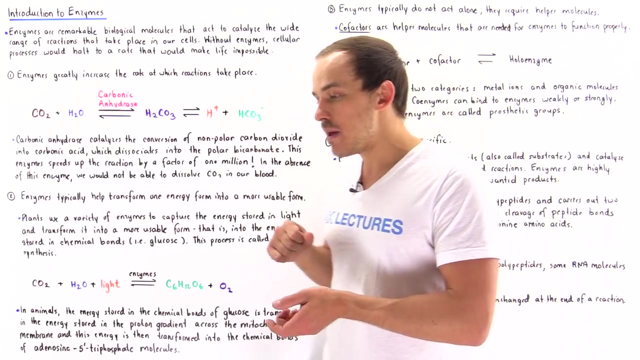 different enzymes that essentially catalyze the transformation of the energy stored in the chemical bonds of glucose into the energy that is stored in the proton gradient that exists across the membrane of mitochondria, And then the energy stored in that membrane in the electrochemical gradient due to the protons found across the mitochondrial membrane. 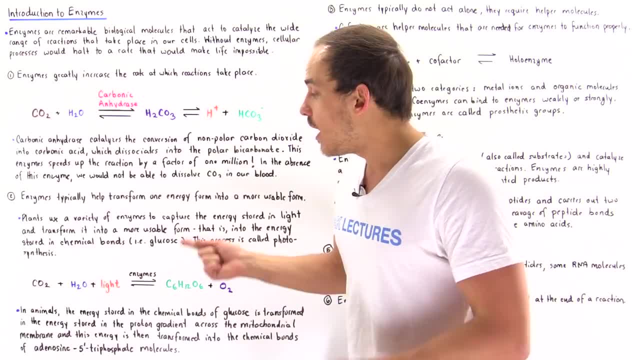 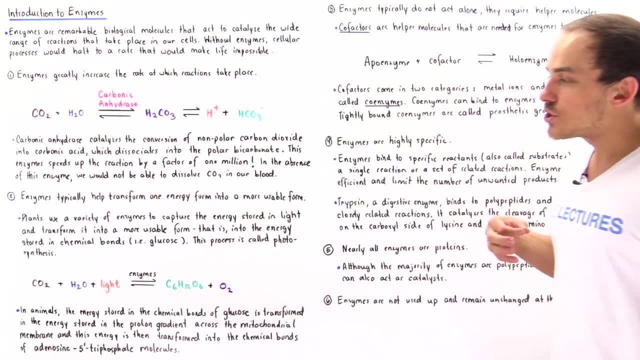 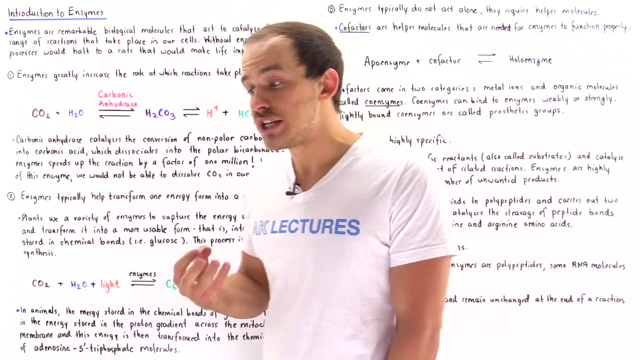 that energy transformed into energy stored in the bonds of ATP molecules- adenosine triphosphates- and we'll discuss that in much more detail eventually. So we see that these enzymes are very, very good at transforming one form of energy that we can't use into a form that we can use, and that is what enzymes do. 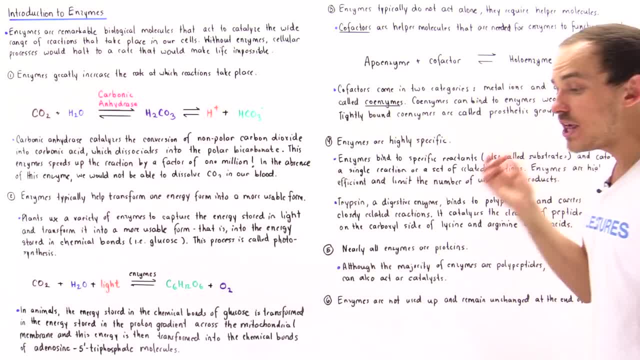 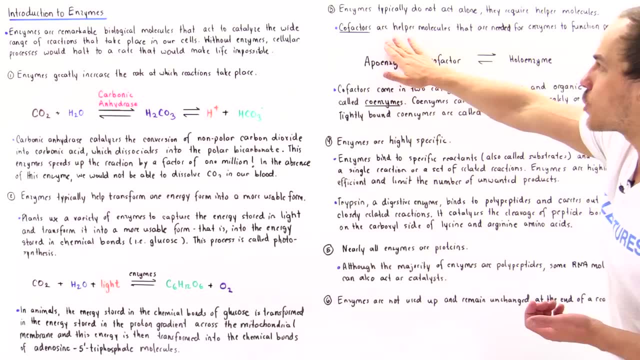 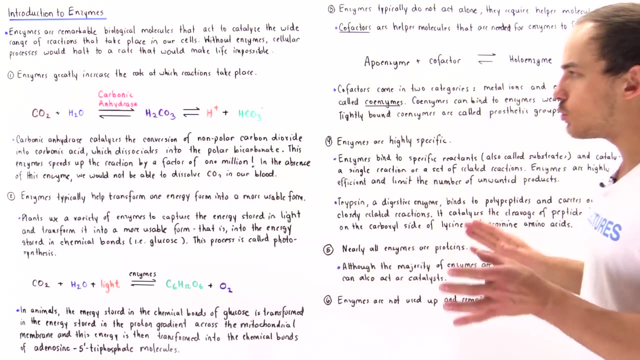 Number three: The enzymes typically do not act alone and they require additional molecules, and these molecules are known as cofactors. So cofactors are helper molecules that are needed for the enzymes to actually function effectively and efficiently. So when an enzyme is not bound to its cofactor, we call the enzyme apoenzyme. but when the 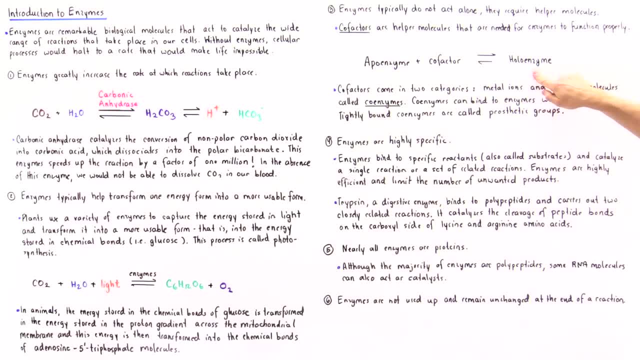 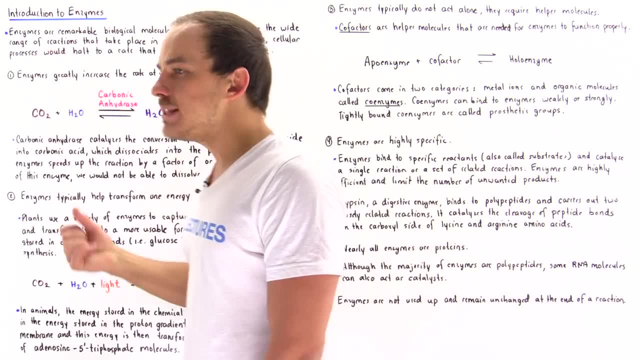 cofactor is bound to the apoenzyme. we call that a holoenzyme. So the holoenzyme is simply an enzyme bound to its cofactor. Now we have many, many different types of cofactors, as we'll eventually see. 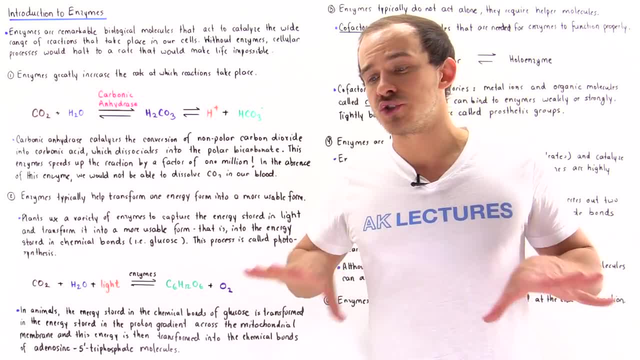 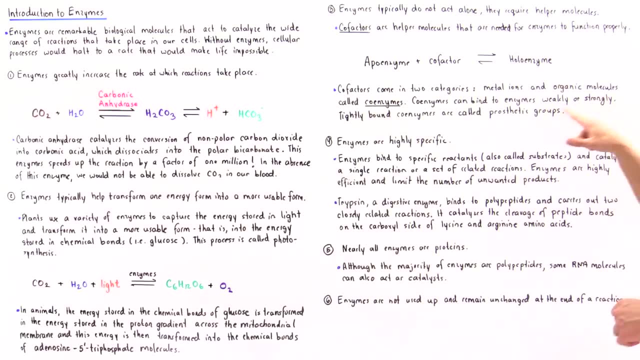 But we can categorize cofactors into two groups, into two categories. We have metal ions and we also have organic molecules known as coenzymes, that are usually formed from vitamins. Now, one example of a metal ion that acts as a cofactor for coenzymes is a coenzyme of 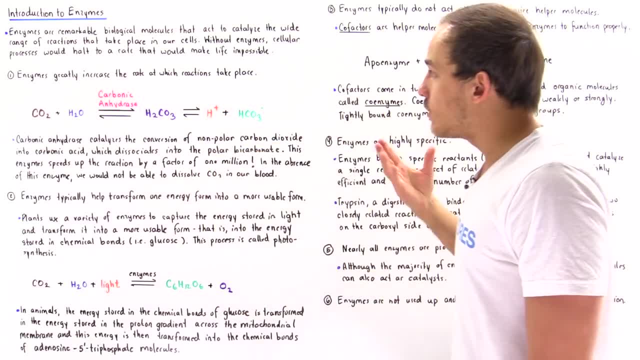 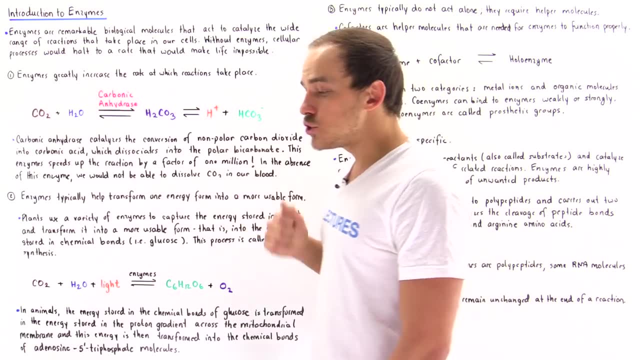 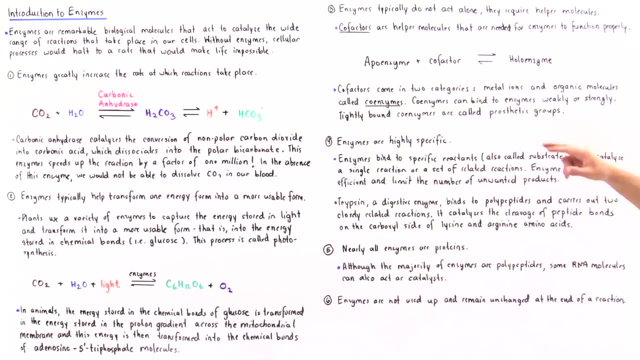 carbonic anhydrase, which is the zinc atom, And we'll talk about that in detail in a future lecture. Now, coenzymes can bind onto proteins either strongly or weakly, And if we have a coenzyme that is bound very tightly to the enzyme, that is known as a 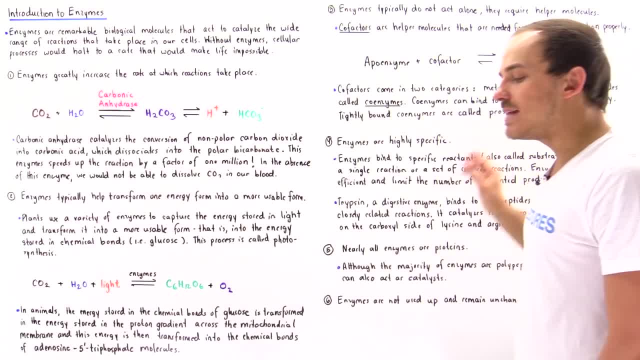 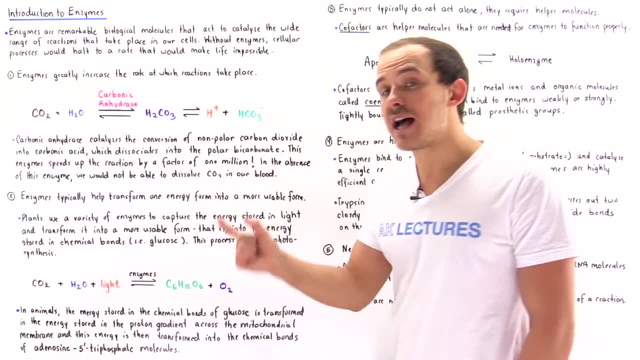 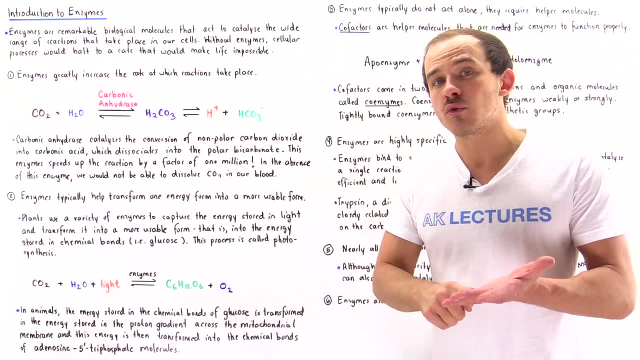 prosthetic group Number four, enzymes are extremely efficient and extremely specific molecules, And what that means is enzymes only bind to specific substrate, specific molecules, and they carry out either a single reaction or a set of reactions that are closely related to one another. 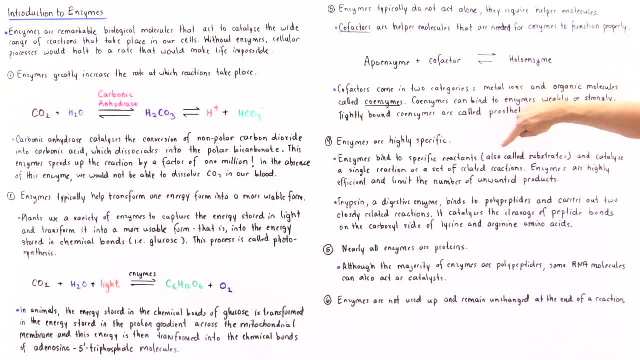 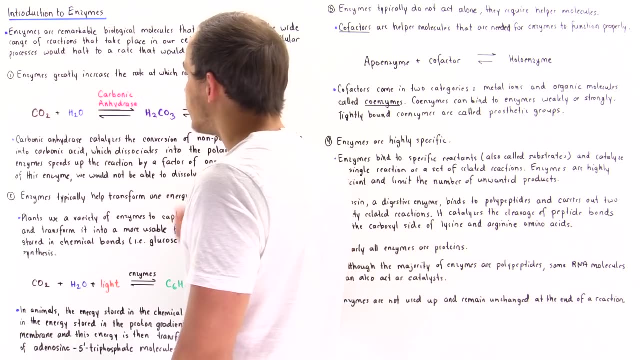 So enzymes bind to specific reactants- we also call substrates- and catalyze a single reaction or a set of related reactions, And enzymes are highly efficient and limit the number of unwanted products, For example, in the case of carbonic anhydrase. carbonic anhydrase binds the CO2 and the 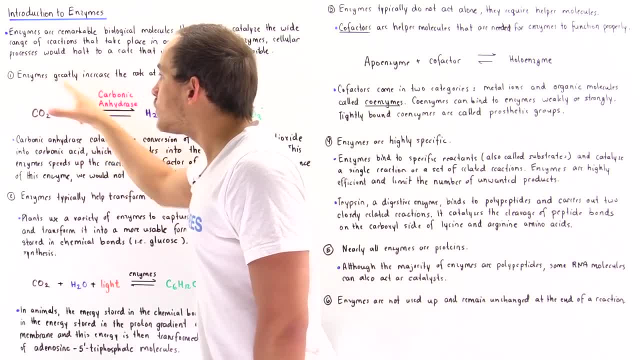 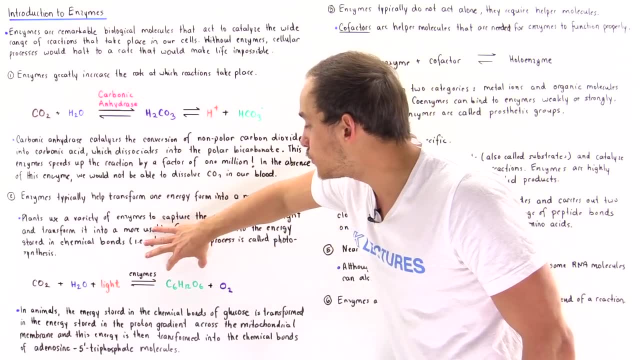 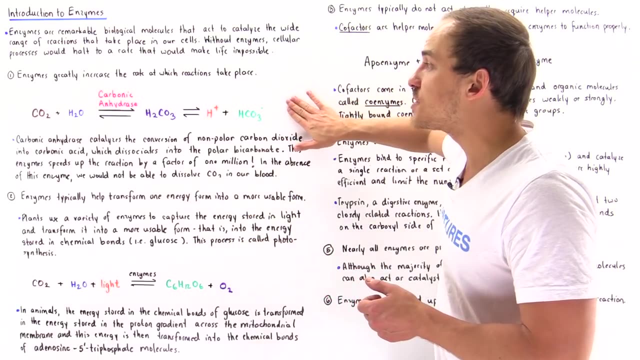 water and the CO2 is the substrate. Now, CO2 can react with water in many different ways. For example, in this particular case, we saw that we can produce sugar molecules and oxygen molecules, and these are unwanted products, at least in this particular case. 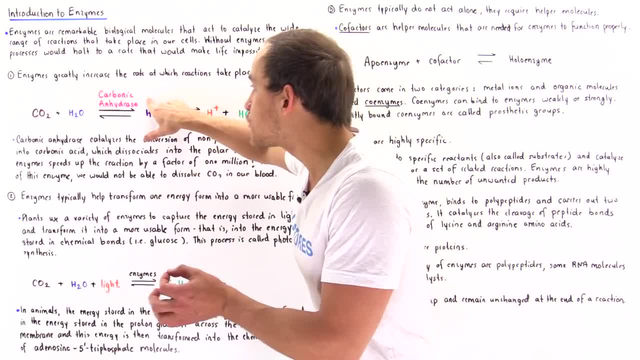 So what carbonic anhydrase does is it ensures that the carbonic anhydrase is a very strong reaction to water. So you see where our reaction is not a silver lining. you see where our reaction is a combination of water, fat and oxygen and carbonic anhydrase and carbonic anhydrase. 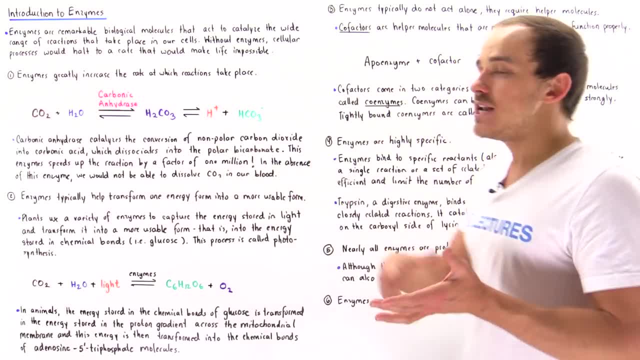 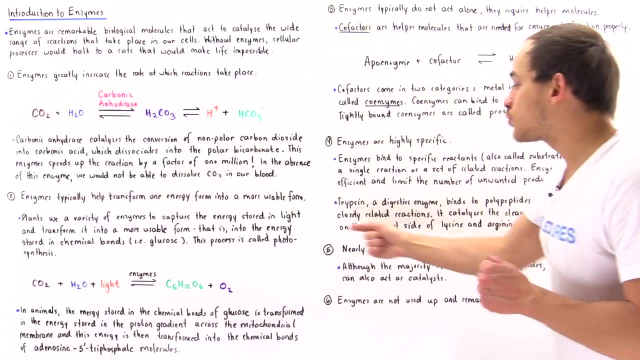 It is just a matter of increasing the amount of oxygen that gets produced by carbonic anhydrase. Now, carbonic anhydrase system does not do much to cause our water to stick to whatever substance we have combined with it. Again. so table 1 for this experiment. we say that carbonic anhydrase has a childhood. 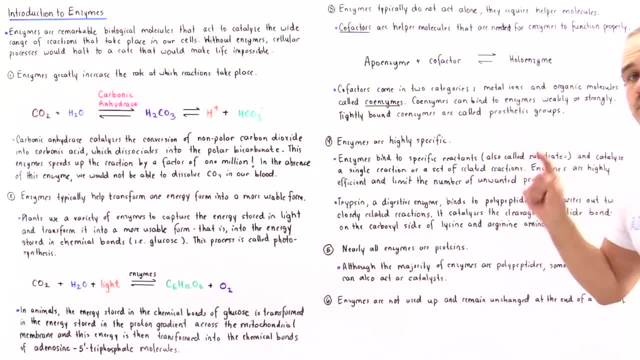 process called angina- Now, this is a rustic name for a result of being able to be combined withこれは, And it was from that concrete foundation I have trapodate. that appeared ingest into our body, and it basically carries out a set of two closely related reactions. 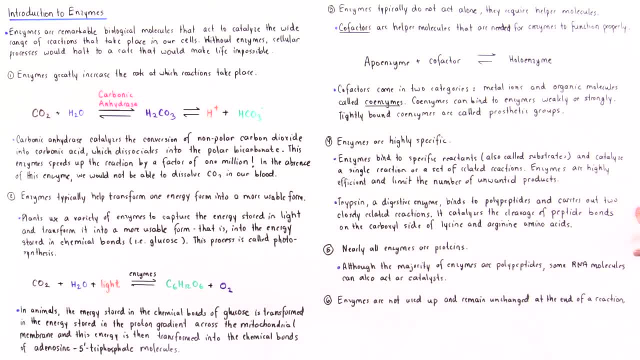 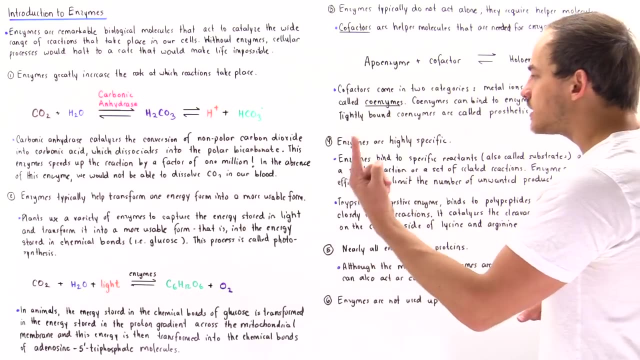 In one of the reactions it basically cleaves peptide bonds on the carboxyl side of lysine. In the other reaction it binds and cleaves on the carboxyl side of the arginine amino acid. So this trypsin has a single type of substrate, namely the polypeptide, and it carries out. 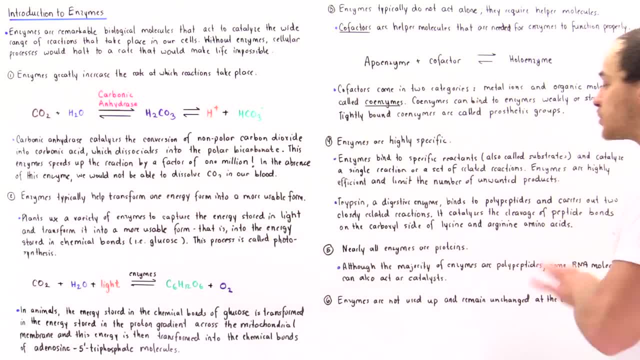 two sets, two types of very similar reactions. In one reaction, it cleaves lysine on the carboxyl side. In the other reaction, it cleaves arginine on the carboxyl side. Number five: nearly all enzymes are protein. 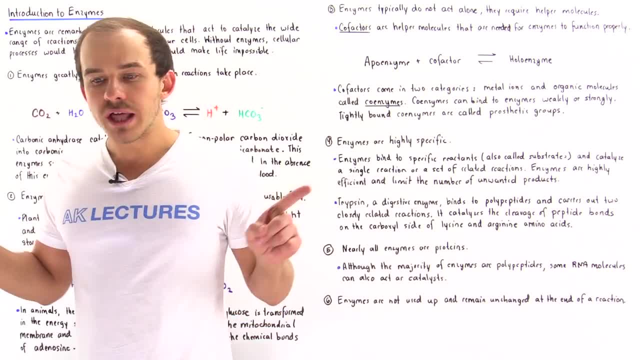 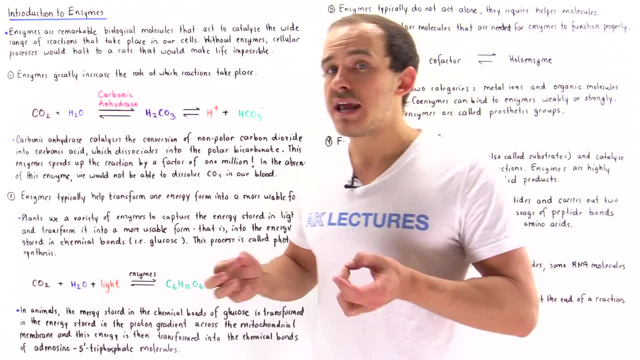 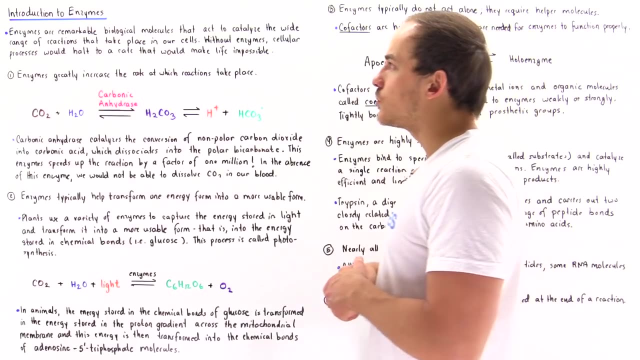 So long ago, we essentially thought that all enzymes were protein, But now we know that some enzymes are actually RNA molecules. So RNA molecules, certain RNA molecules, also have the ability to catalyze reactions, as we'll see eventually. And the last thing we're going to mention about enzymes is: enzymes are not actually. 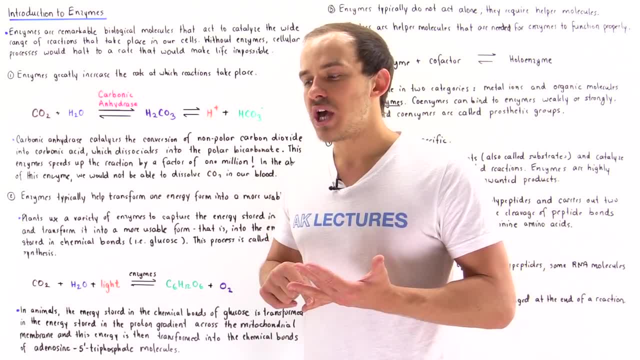 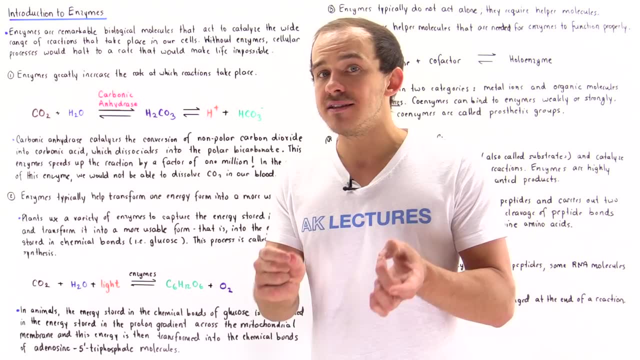 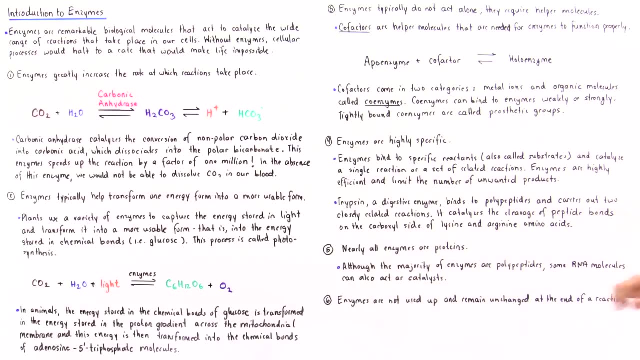 used up are not depleted in chemical reactions. And if enzymes are changed or altered in some way in the reaction, at the end of that reaction the enzyme will change. It will assume its original shape and original structure. So enzymes are not used up and remain unchanged at the end of the reaction. 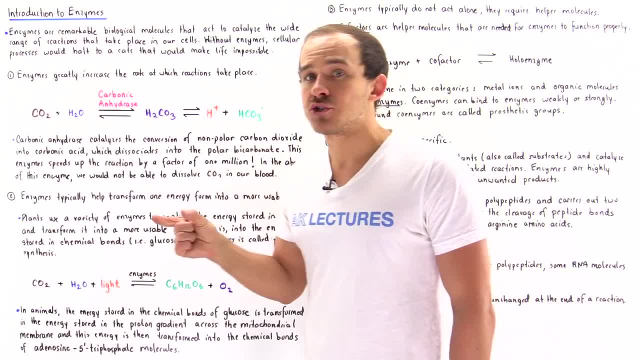 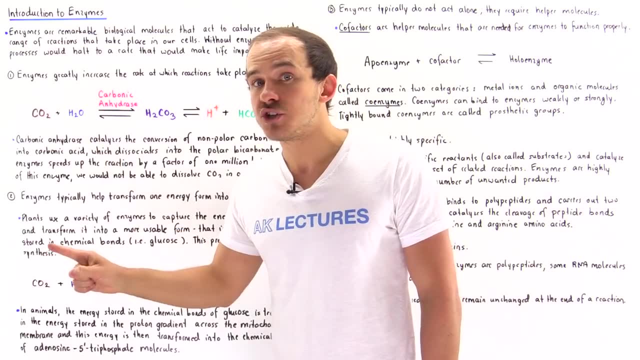 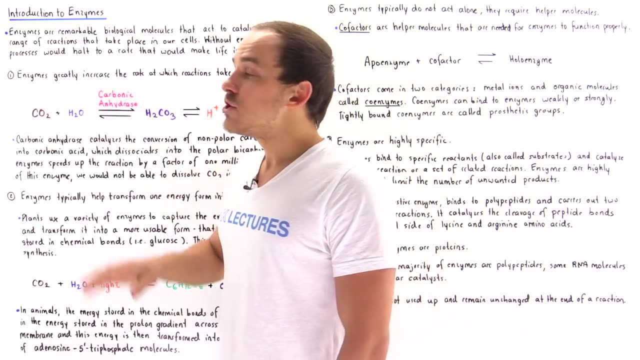 Now this is not to say that enzymes during the reaction aren't changed in some way. They might be changed, Their structure might be changed, But at the end of the reaction, when the enzyme releases the substrate, it assumes its original structure and its original shape. 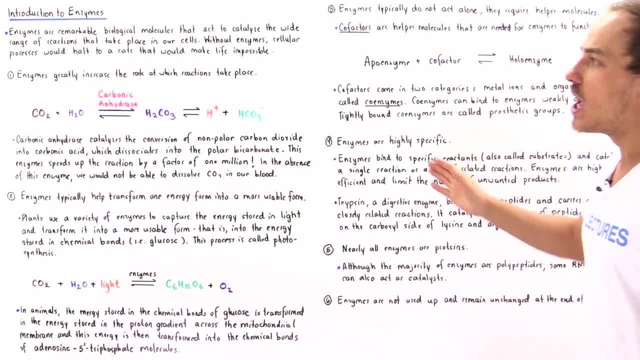 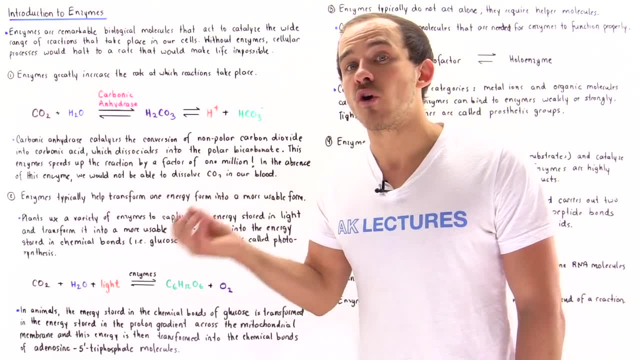 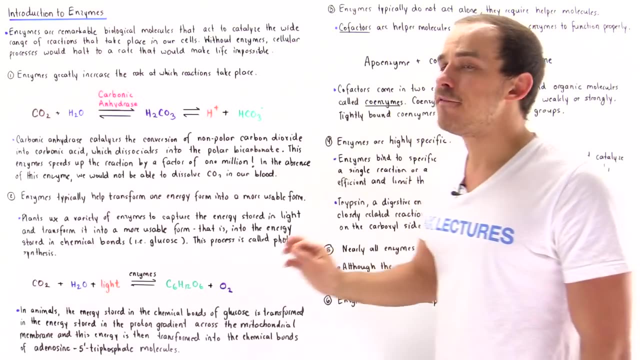 So these are the six facts You have to remember about enzymes. Enzymes greatly increase the rate at which reactions take place. Enzymes typically help transform one form of energy into a much useful form of energy. Three enzymes do not function alone. 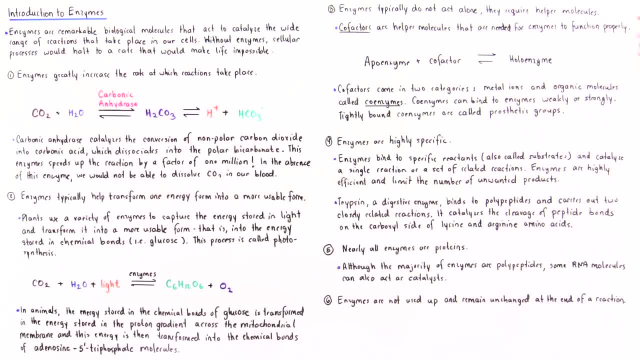 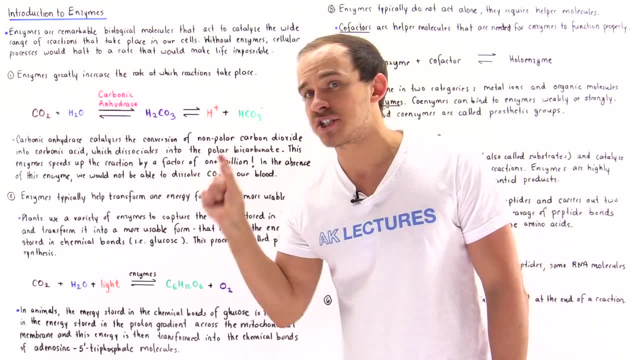 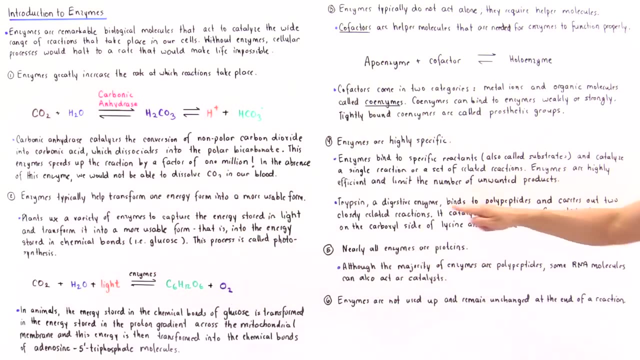 And they typically do not And they typically need these helper molecules we call cofactors. Number four: enzymes are highly specific. They bind specific substrates. They bind specific substrates. They do not come in one single reaction or a set of reactions that are similar. 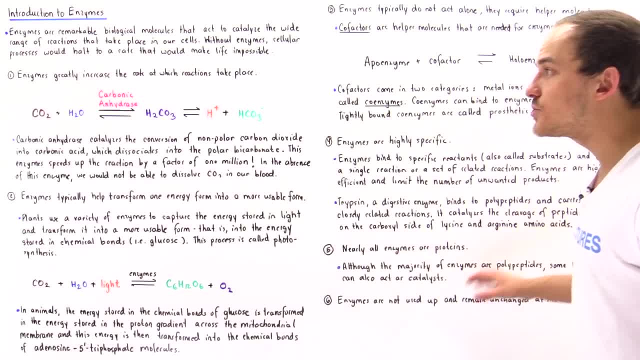 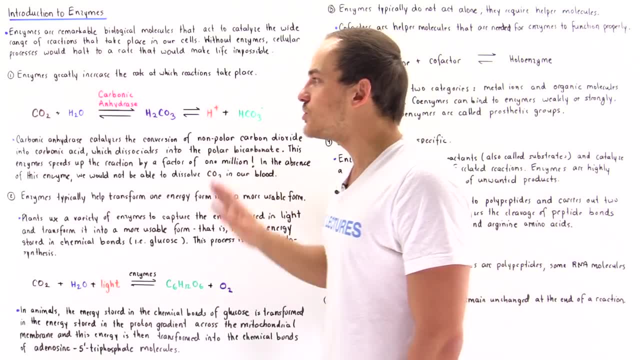 Number five: nearly all enzymes are proteins. Some enzymes are RNA molecules. And number six: enzymes are not depleted. They are not changed At the end of the reaction. they remain exactly the same. 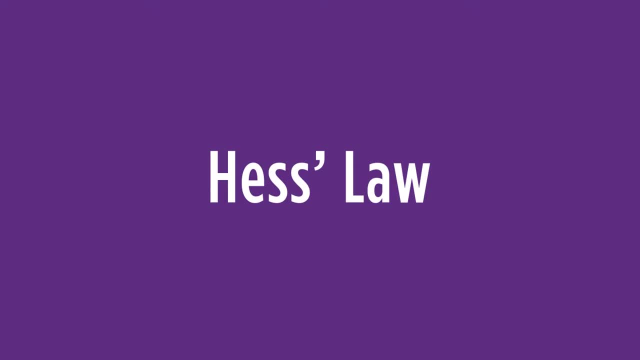 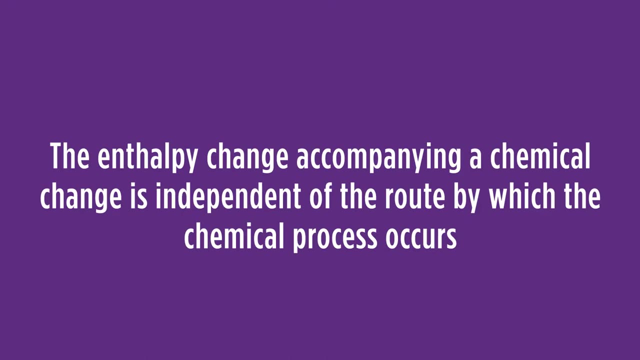 In this video we're going to look at Hess's law. Hess's law states: the enthalpy change accompanying a chemical change is independent of the route by which the chemical process occurs. Hess's law is used to calculate delta H for a reaction when we don't actually have the